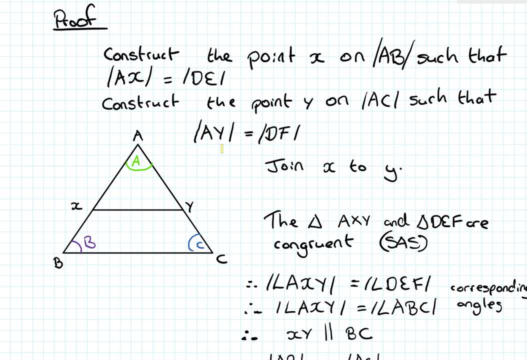 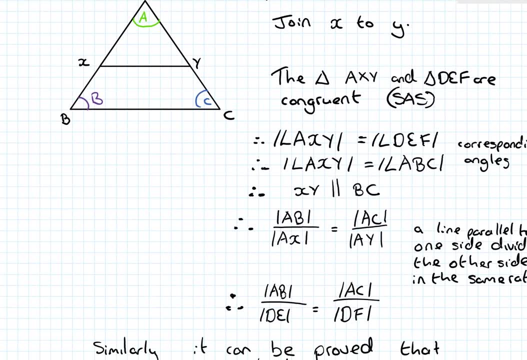 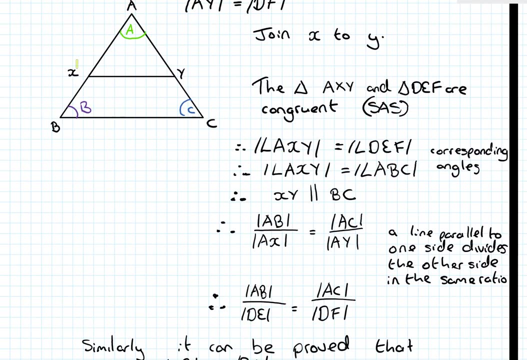 The angle A is common And this length is also equal to the other one, which was DF. We know, then, We know that the angle AXY, So AXY, this angle here Is equal to the angle DEF, which was on the previous triangle, as it was corresponding to it. 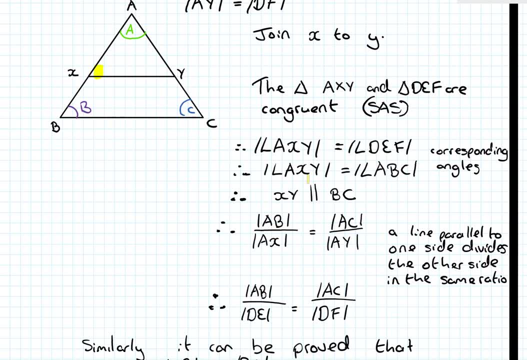 We know that this length here AXY is equal to ABC, here ABC, so it's equal to here as corresponding angles. We know the length XY is parallel to BC. We know that this length here AXY is equal to DEF, because they're congruent triangles. 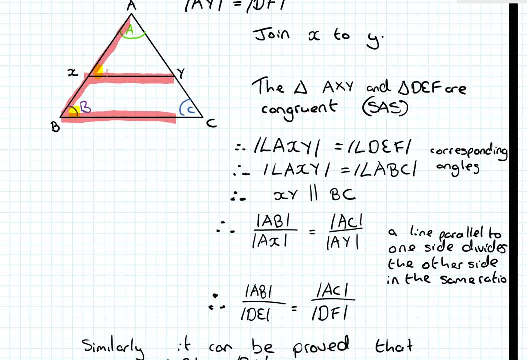 We know AXY and ABC, this angle here and this angle here have to be the same, As we knew that they were congruent triangles, the triangles ABC and DEF, So that That implies, then, that these lines are parallel, as those two angles are the same. 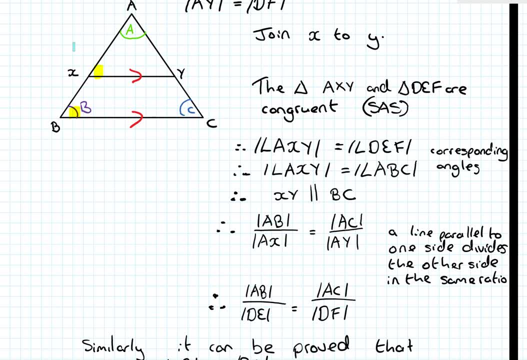 Then we know that the ratio of A over B is equal to A over X and the ratio A over C is equal to A over Y. The lines parallel to one side divides the other lines in the same ratio, which was theorem 12, that we just proved. 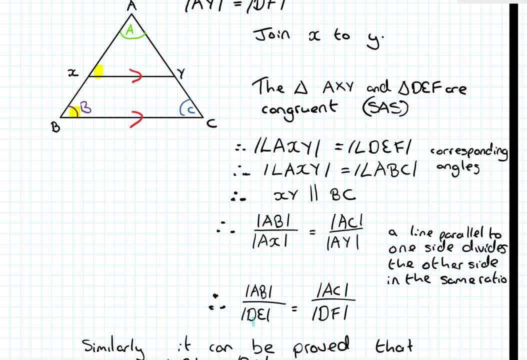 We also know, then, that the length AB is equal to AB over DE- Remember, AX is the same as DE, And we know that the length AY is equal to DF. So it's the same piece of maths, it's the same line. 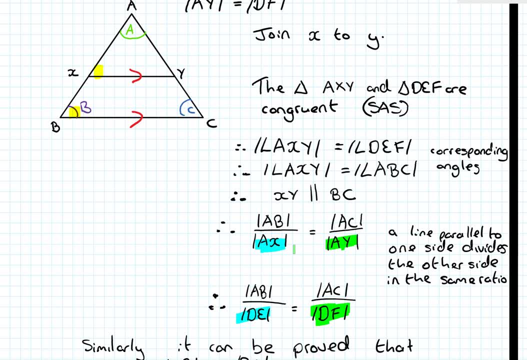 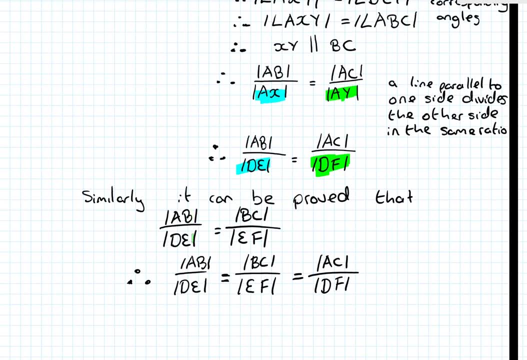 But yeah, we're now talking about the two congruent triangles. From that we can also just say: similarly, We proved that the length AB over DE is equal to BC over EF. and write it all out: what was asked. 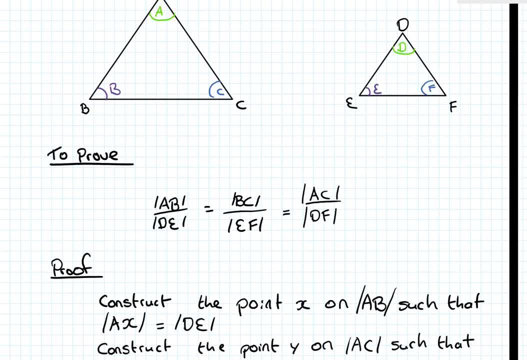 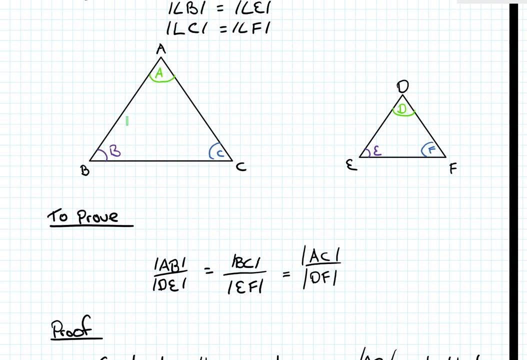 Key points to it, I suppose, is really making sure that you know the construction. what you're going to do, We are going to construct this line across here using similar triangles and then using theorem 12 also.